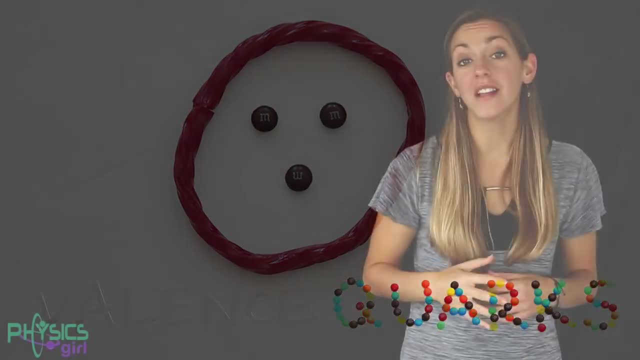 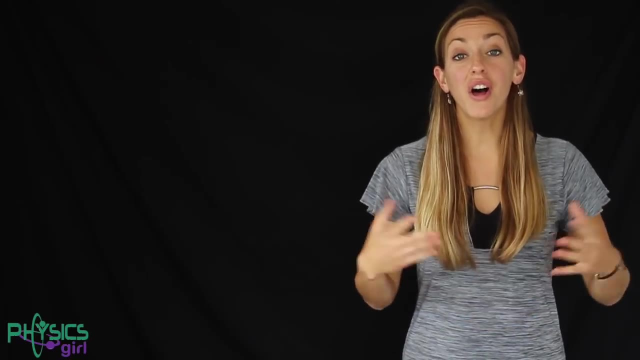 quarks are known as valence quarks and they're definitely there, But the proton could have an additional up quark, anti-up quark pair. An anti-quark is the anti-particle of a quark And it could have other types of quarks: pairs of strange quarks and anti-strange quarks. charm quarks and anti-charm quarks. In fact the proton likely has tons of quark-anti-quark pairs, But there's more. The quarks are held together by the strong force which is carried by particles called gluons. So inside the proton there, 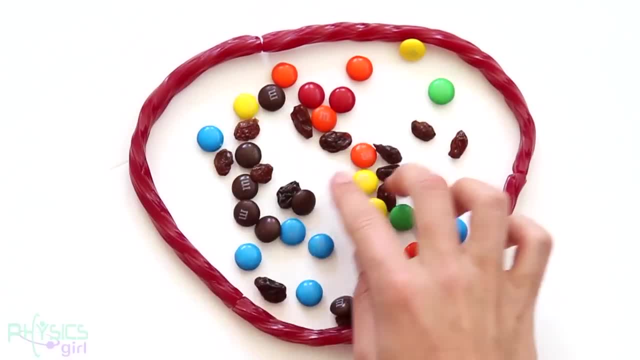 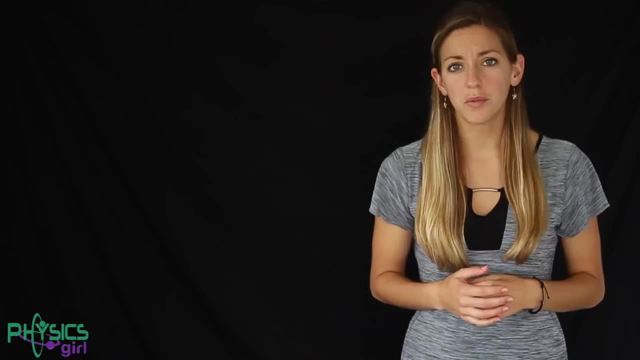 are zillions of gluons and quarks all zooming around close to the speed of light and colliding and annihilating, And new ones are forming And it's a crazy raging party, such as the quantum world in a proton. Wouldn't that violate some kind of conservation law if particles 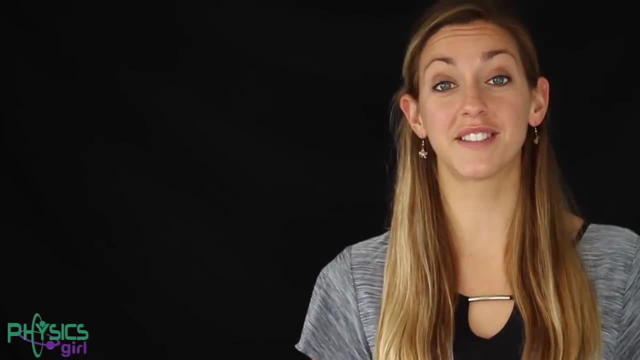 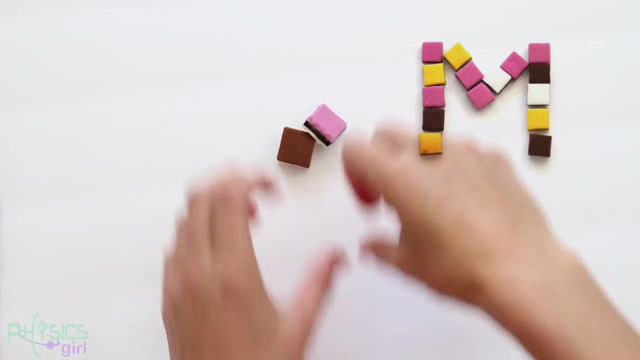 just appeared. in the proton, Quarks can and do just appear and disappear, but not out of nothing. Einstein's famous equation E equals mc squared means that mass can turn into a lot of energy, Or a lot of energy can turn into mass. In fact, the quarks that comprise a proton only. 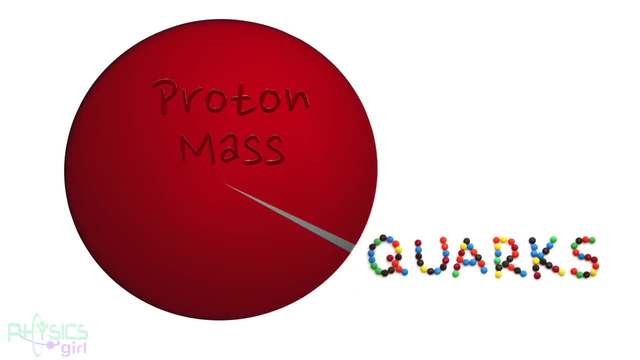 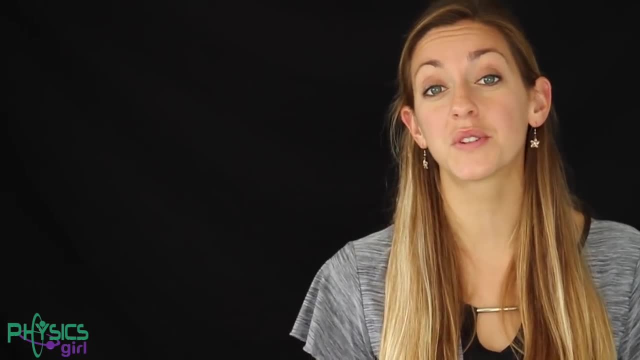 make up 1% of the total mass of that proton. That's like saying I drop some quarters in a bag and suddenly it weighs 10 pounds. There's a lot of energy in all the motion of those crazy partying particles, Particles. 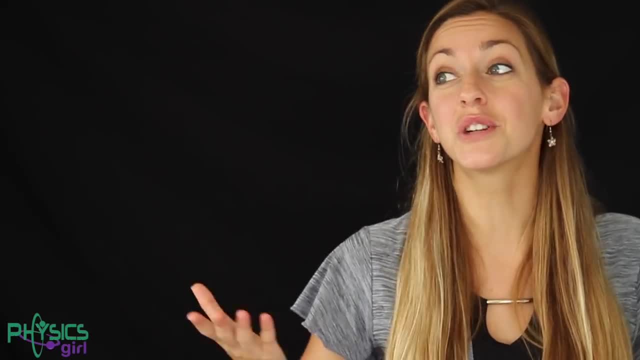 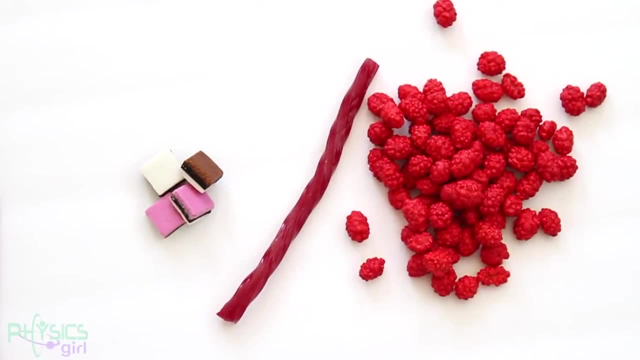 And there's energy in the gluon field. All of this energy contributes to the mass of the proton. E equals mc squared. All we need to conserve is the total mass energy of the proton, and nothing is violated as quark-antiquark pairs pop in and out of existence. 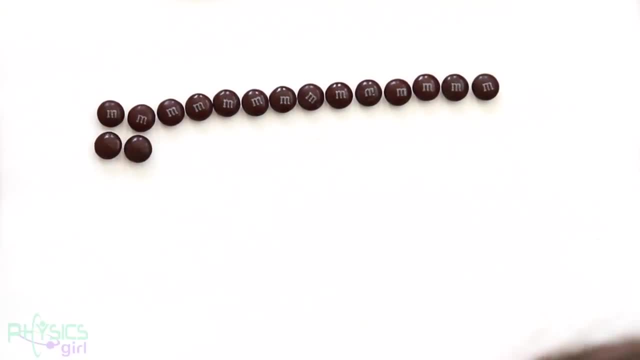 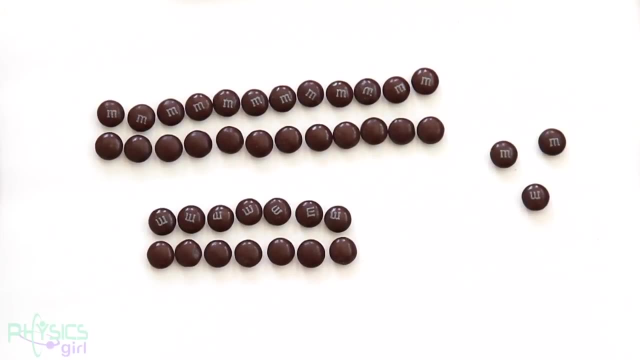 But there are a few other constraints: The total number of up quarks must be two more than the anti-up quarks, and there must be one more down quark than anti-down quarks, so that the valence quarks come to a total of three And the quark-antiquark pairs of other types must all cancel out, Like the top quark and the charm quark and the strange quark and the bottom quark. When quark pairs spontaneously appear in the proton, they're called quark-antiquark quarks. 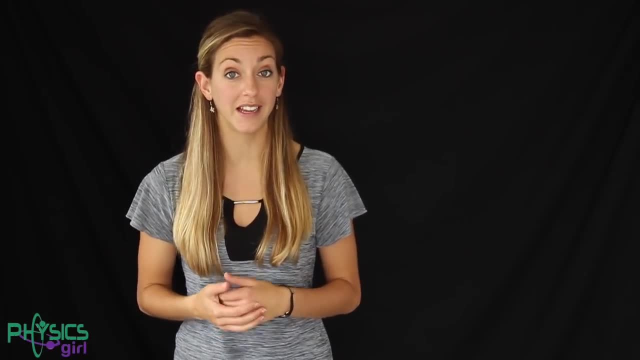 They're called quark-antiquark quarks And on other properties must be conserved as well, like charge. So if a quark with charge positive 2 thirds appears, its partner must have charge negative 2 thirds And the spin. 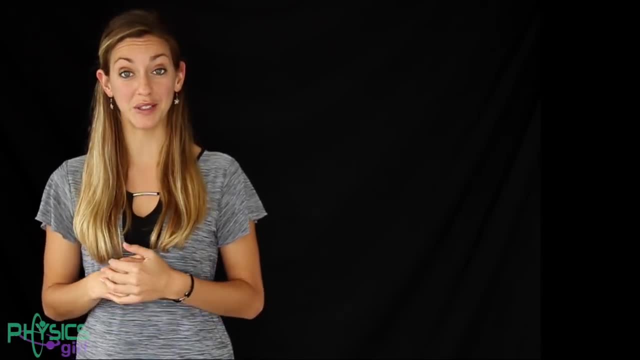 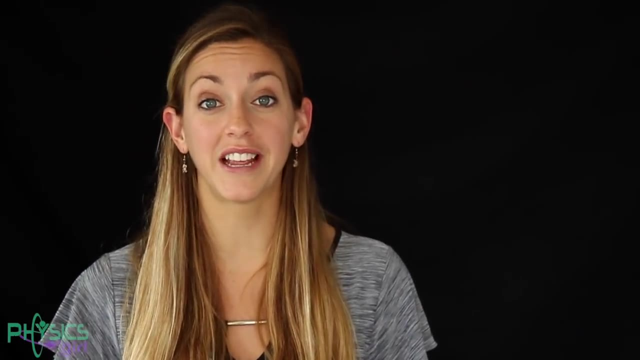 of the particles must be opposite and the colorlessness of the proton must be conserved. This is cool. Quarks all have color, except it's not like real color. Color in quarks is a type of charge like the electric charge, except instead of the electromagnetic force. 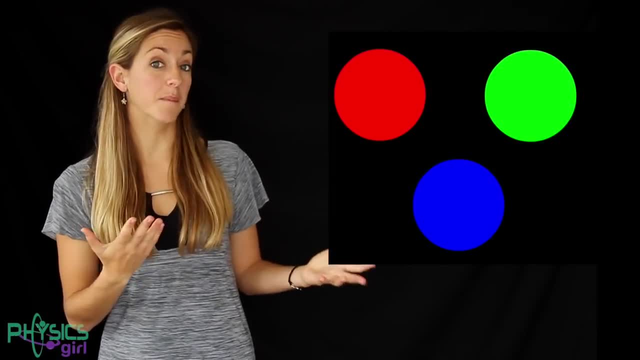 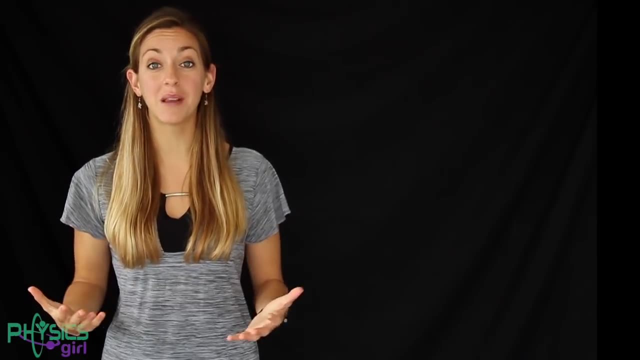 it corresponds to the strong force. Quarks can be red, green and blue, like the three primary colors of light, And when you mix those colors You get white light. So when I said that protons are colorless, that means that their three